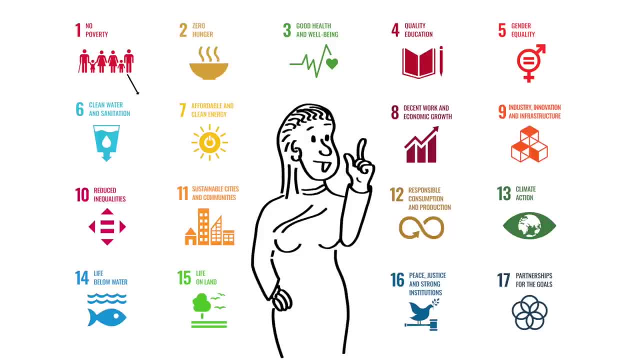 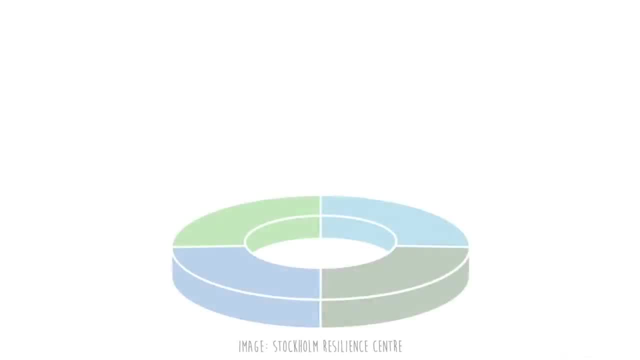 becoming sustainable, Or do they? First, let's look at how they are interconnected instead of looking at them individually. The Stockholm Resilience Centre suggested organizing the SDGs into three layers: The environment as the foundation. supporting society, which supports the economy. 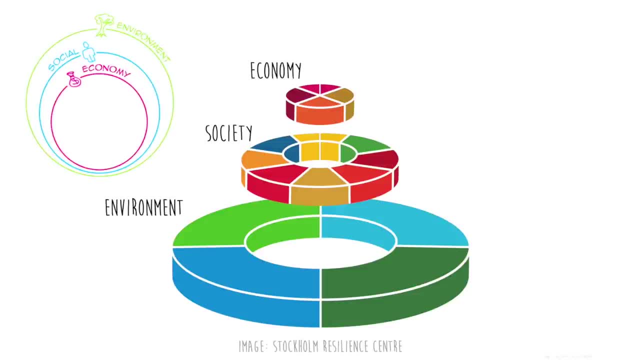 This is like the triple bottom line or the three pillars of sustainability. The SDGs are the three pillars of sustainability that I presented in another video. I put a link in the description below. Essentially, sustainability is about meeting human needs within ecological constraints, and the economy is a strategy to make money while achieving sustainability. 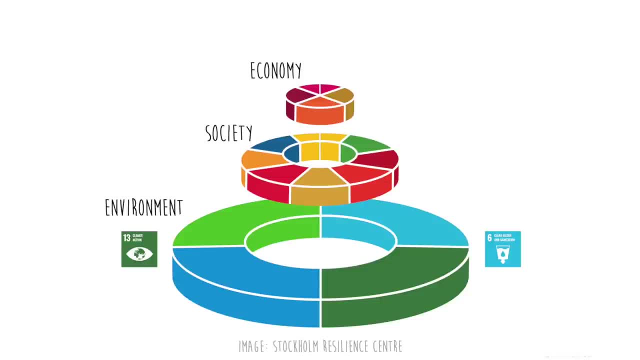 There are four goals about the environment, Clean water, climate action, life on land and life below water. Eight goals are about society: No poverty, zero hunger, good health and well-being, quality education, gender equality, affordable and clean energy. 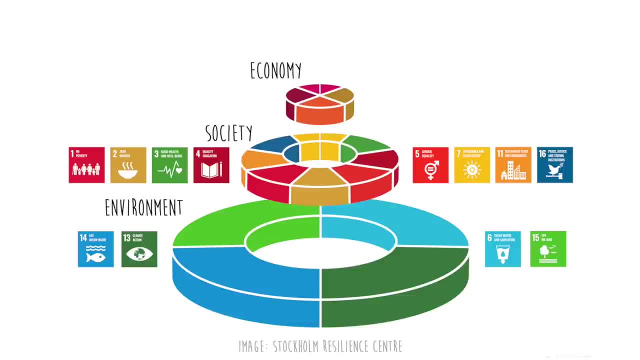 sustainable cities and communities, and peace, justice and strong institutions. And these four goals are about the economy: Decent work and economic growth, industry, innovation and infrastructure, reduced inequalities, responsible consumption and production. They call this representation the SDG World. 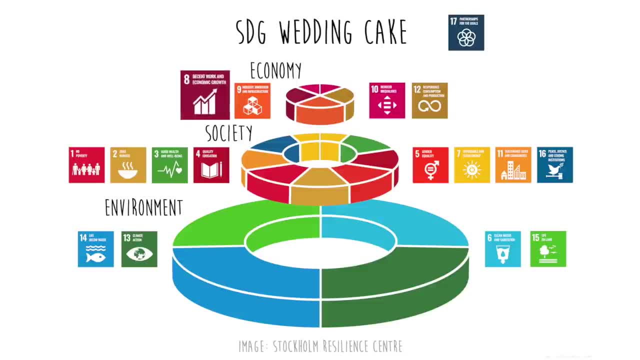 Wedding Cake. In other words, we can't achieve decent economic growth or even food security without first taking care of our oceans. as was demonstrated in Newfoundland during the collapse of the Atlantic cod fisheries in the 1990s And to use the more recent example of the coronavirus crisis, we can't have everybody. 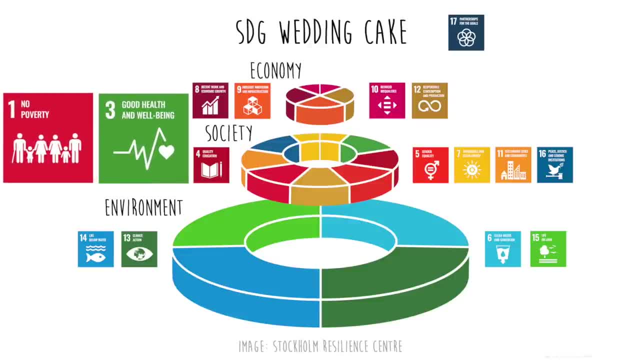 in good health and achieve no poverty without taking care first of our land, forests and our greenhouse gas emissions. We can't have everybody in good health and achieve no poverty without taking care first of our land, forests and our greenhouse gas emissions. 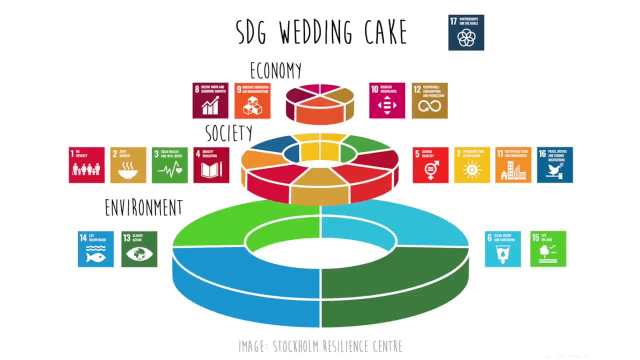 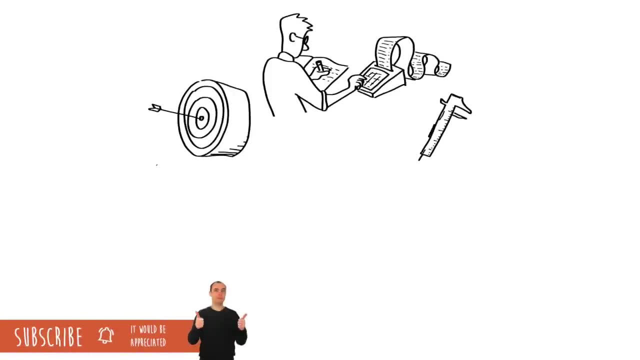 My video on coronavirus explains this in more details. With the 17 goals come targets and indicators. I am not going to bore you with all the 169 targets and 232 indicators, but if we look at the affordable and clean energy goal as an example, 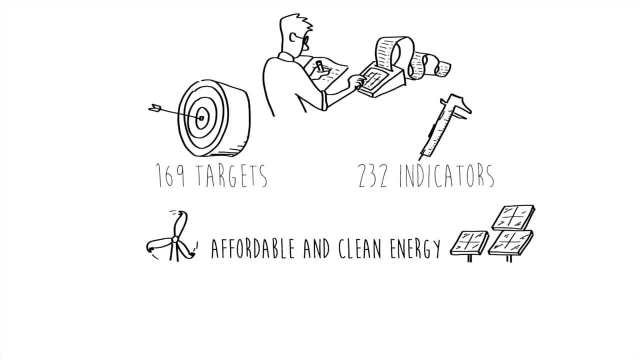 it has five associated targets which read like this: By 2030, ensure universal access to affordable, reliable and modern energy services. By 2030, increase substantially the share of renewable energy in the global energy mix. By 2030, double the global rate of improvement in energy efficiency, etc. 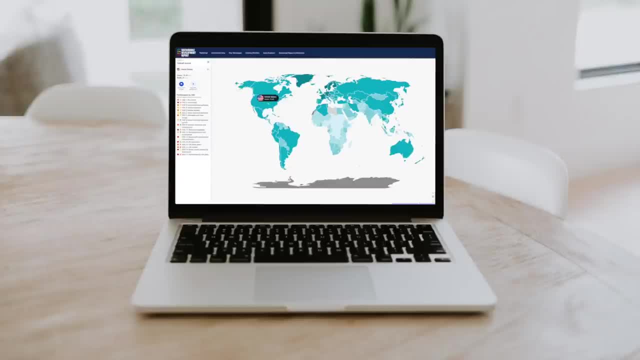 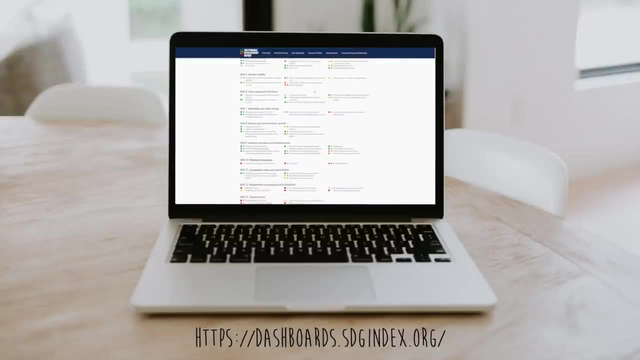 And we can look at the performance of each country by indicator on this website. It looks like this for the United States, for instance: If a country is doing well on the SDGs, does that mean that they are more sustainable? Let's look at the top of the list. All these indicators indicate that they are more sustainable. 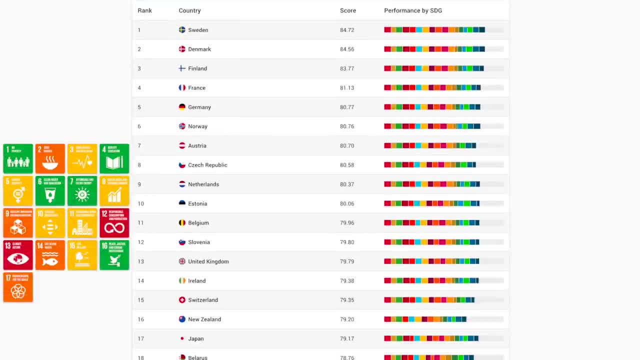 Let's look at the top of the list. All these indicators indicate that they are more sustainable. All these indicators indicate that they are more sustainable. These European countries are doing really well on poverty, health, education, etc. But they also have some of the largest ecological footprints per capita in the world. 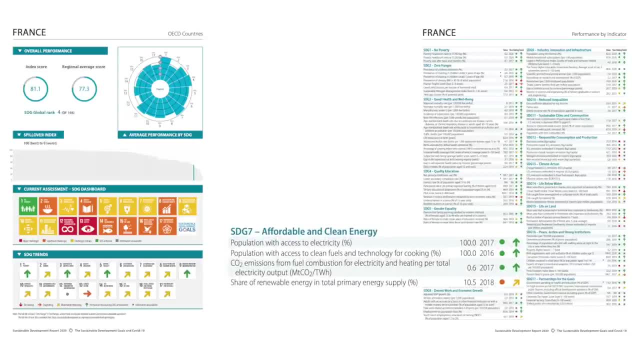 Although it is interesting to look at each individual target and indicator to see how a country is doing on individual goals, looking at the aggregate score of a country can be misleading, as developed countries look better as a whole but tend to use a lot more resources and contribute. 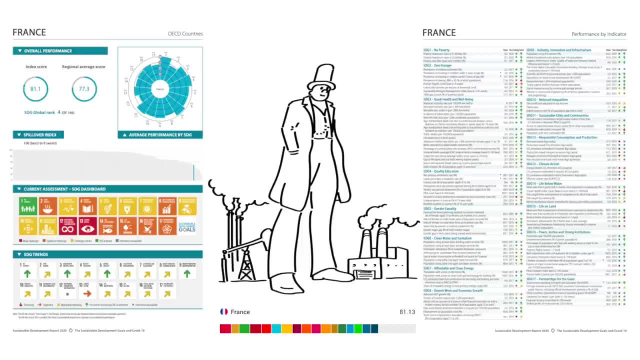 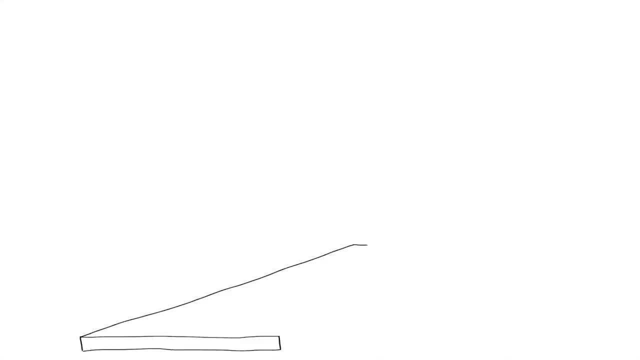 more to climate change To break down sustainable development into all its dimensions. these 17 goals are great, But if you are trying to make a plan for a country to become sustainable, I would recommend using these first-order principles for sustainability that are grounded in science. 3 ecological ones. 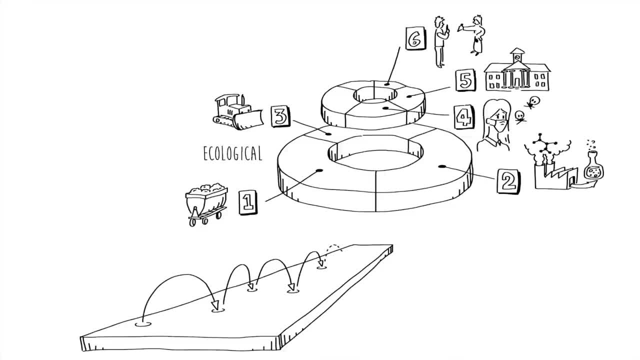 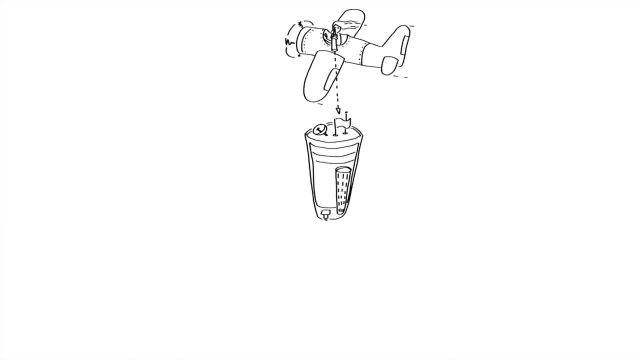 and 5 social ones. They are necessary, sufficient and non-overlapping. Once we comply with these principles, we are truly sustainable. I included the video link in the description below. If you are using these 17 goals to see if your company is becoming sustainable, FutureFit Business offers a holistic 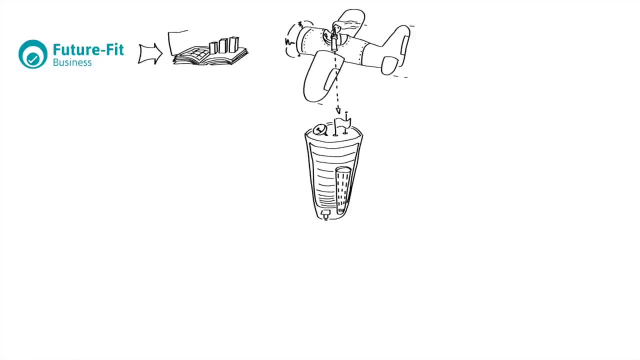 benchmark for companies to assess their social and environmental impact. This benchmark has breakeven goals and positive pursuits beyond the goals that you can organize by SDG or by topic. Let's look at waste, for instance. For waste to not exist anymore, operational waste in the world is not sustainable.